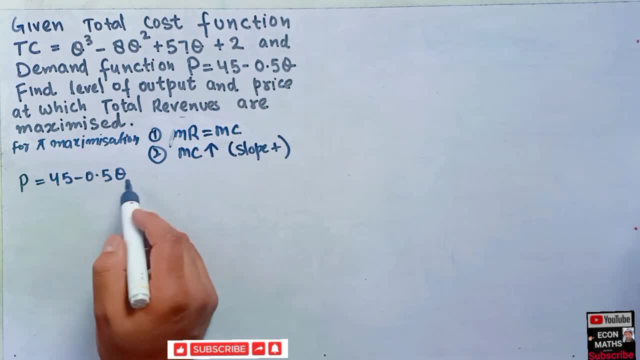 Simply price times quantity. Since this is that this is P, we will multiply it by Q. So total revenue is price times quantity. So price times quantity. So I will write: this is our price function. So I will write 45 minus 0.5 Q And I will multiply it by Q. 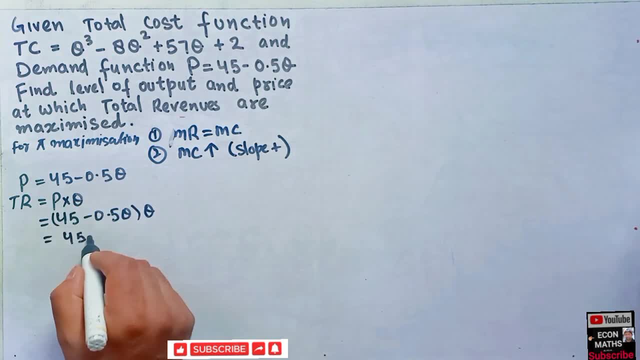 So this becomes 45 minus 0.5.. 0.5 q square. so this is our total revenue. from total revenue we can calculate the marginal revenue. marginal revenue is simply the first derivative of the total revenue with respect to quantity. so our marginal revenue is the derivative of total revenue. so i will write. 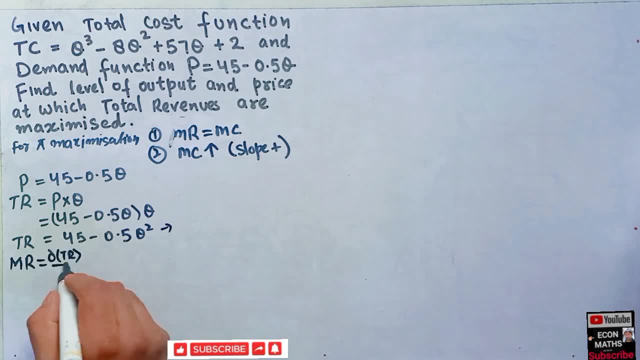 d, dr divided by dq, which is equal to. so sorry, here it is 45. q. now how to find the derivatives? it is very easy. i will not go into the detail here. so here the derivative of q is 1, so 45 into 1 is 45 minus. this 2 becomes coefficient, so 2 into 0.5, which is equal to 1. so we: 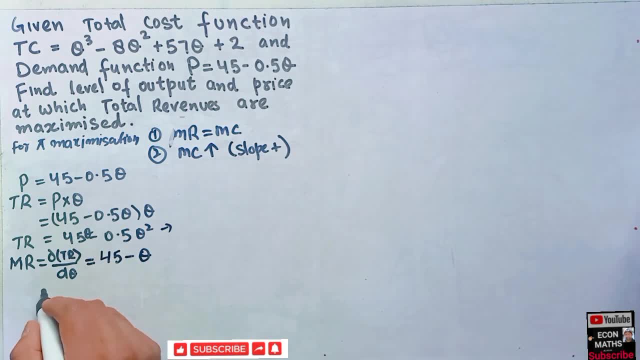 will write the derivative of q as 1. so we will write the derivative of q as 1, so we get q here means our marginal revenue is equal to 45 minus q. this is our marginal revenue. similarly, we will find the marginal cost okay. our first. we are given. the total cost function is given. 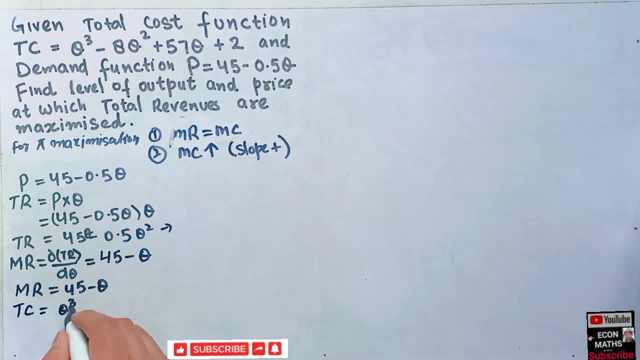 is this very function, that is q cube minus eight, q square plus 57, q plus two. from this total cost function we calculate the marginal cost by differentiating this total cost function with respect to quantity. so marginal cost is simply the derivative of total cost with respect to quantity. 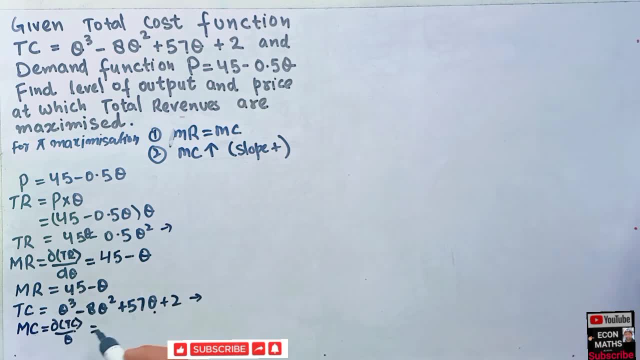 okay, i hope i am making myself clear now we will differentiate this very function. first of all, the derivative of q cube is simply this: 3 becomes coefficient q, and we subtract 1 from the exponent. so 3 minus 1 is 2, so this becomes 3 q square minus. similarly, this 2 becomes coefficient, so 2 into 18 is equal to 16. 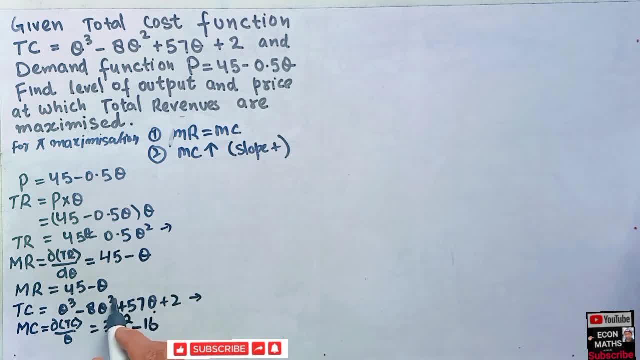 so this is 16. now subtracting exponent by 1, 2 minus 1 is 1, so we will get 16 q. similarly, the derivative of q is 1 here by using the similar logic. so we get here 57 into 1, which is 57. 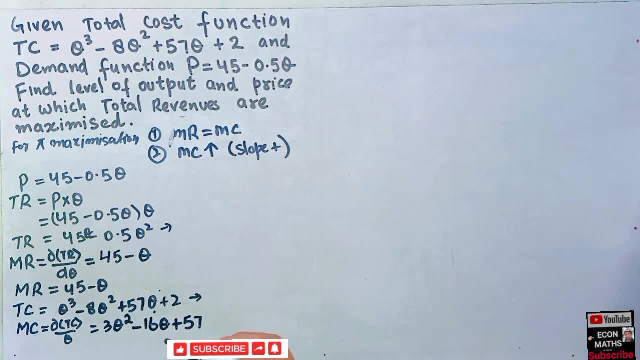 plus the derivative of constant is 0. okay, so this is our marginal cost. now we will use the conditions for profit. so we will use the conditions for profit- sorry, revenue maximization- here. so first condition is: our marginal revenue should be equal to marginal cost. now our marginal revenue is this very function and this is our marginal cost. so we 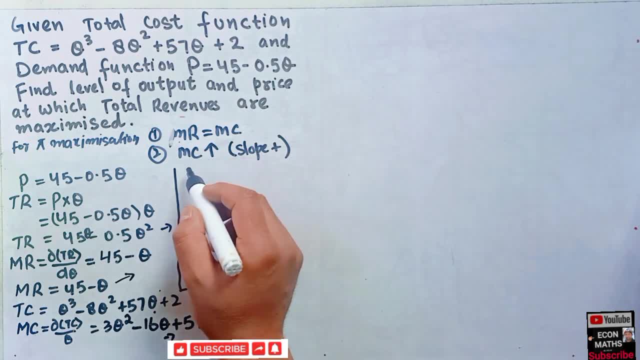 will equate these two functions. so first order condition requires marginal revenue should be equal to marginal cost. okay, so our marginal revenue is this: 45 q, 45 minus q is equal to our marginal cost. is this: 3 q square minus 16 q plus 57. okay, now we will solve this very. 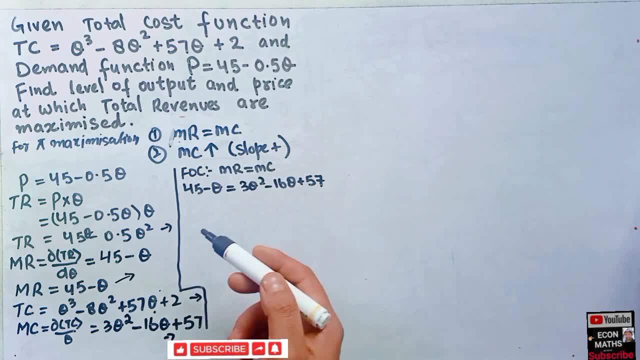 expression for quantity. so just rearranging the terms. so this is your 3 q square. so i will write here: 3 q square. we have a minus 16 q, this is 16 q, this 16 q, and we transpose this here, this will become q. 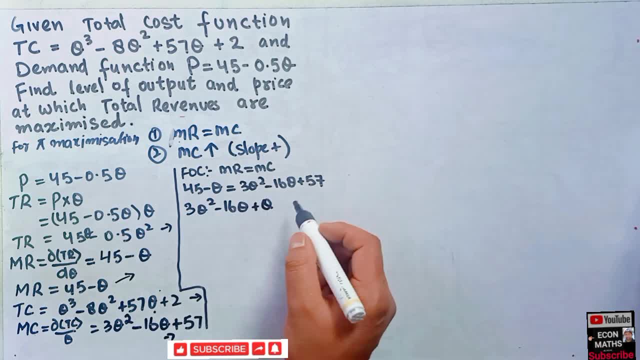 also. now we have 57, 57. now transposing this will become minus 45, okay, and it is equal to 0. so solving this, this is 3q squared now minus 16 q plus q is 15 q. so I will write: minus 15 q, now 57 minus 45, which is: 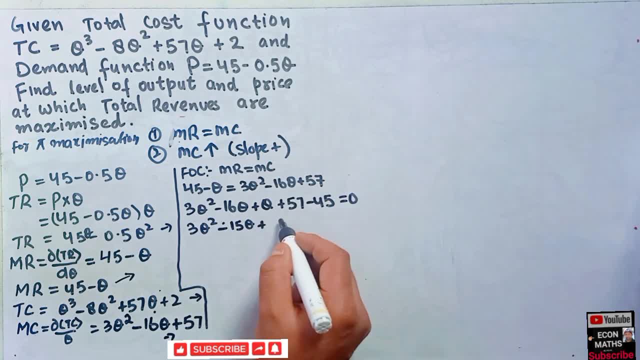 equal to 7 minus 5 is 12- sorry, this is 2, and here 5 minus 4 is 1. so we get this very quadratic equation. now again, solving this, factoring 3 out, so we will get q squared minus 5q. 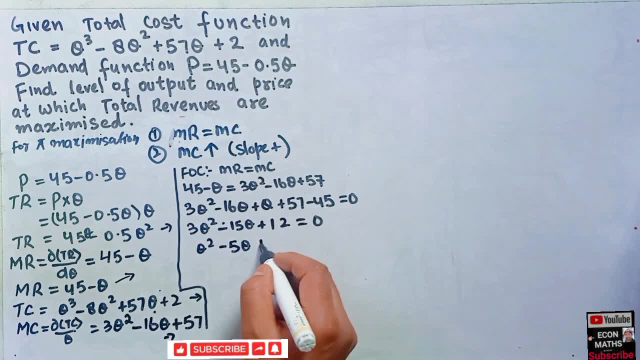 plus 4 is equal to 0. now we have a quadratic equation. how to solve this? we should, so I will just make sure that you get this. we should get two numbers, such that we should get two numbers, such that we should get two numbers, such that we should get two numbers. 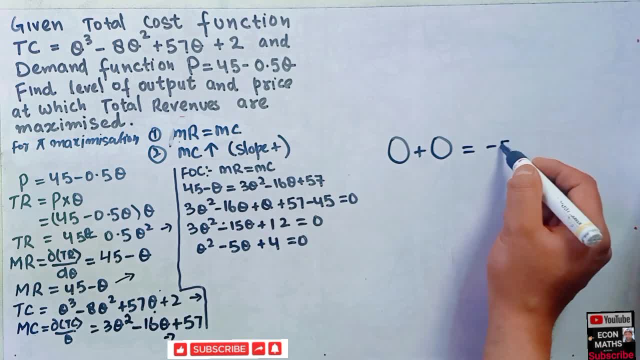 there, some should be equal to the coefficient of middle term, that is minus 5, and the product of those very numbers should also be equal to the constant, that is 4. so if we write here minus 4 and minus 1, so minus 4 and minus 1 is minus 5. minus 4 times minus 1 is plus 4. 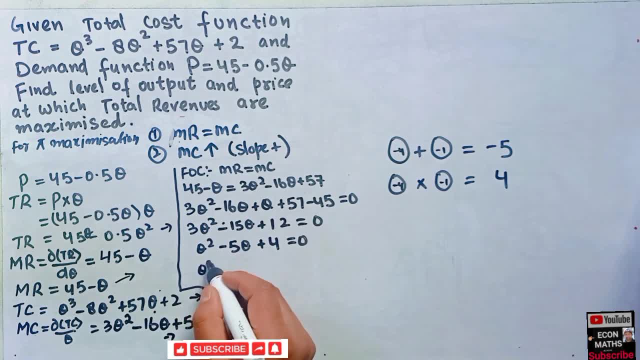 so we get the numbers here. so I will write here q squared. in place of minus 5q, I will write minus 4, q minus 1. q is minus q, and in place of this 4, I can write minus 4 times minus 1. it should. 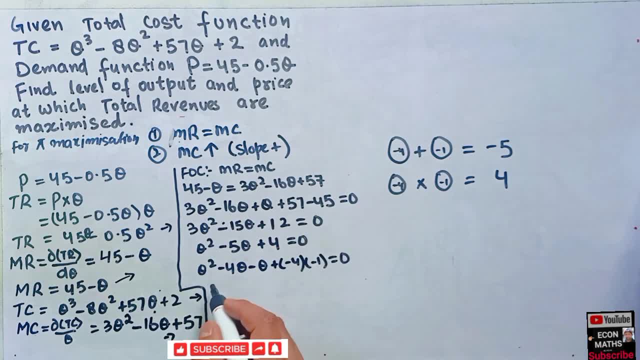 be equal to 0. now making peers here. so this is q, q minus 4 here, factoring minus 1 out and from these very terms, so we get minus 1 out. so we get here: q minus 4 is equal to 0. again, solving q. 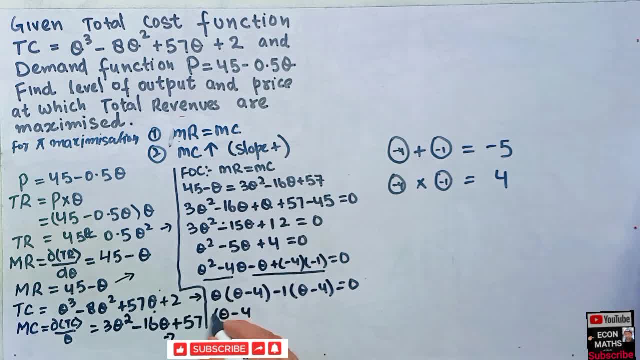 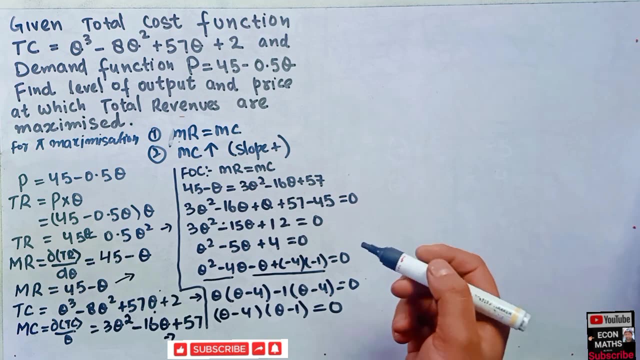 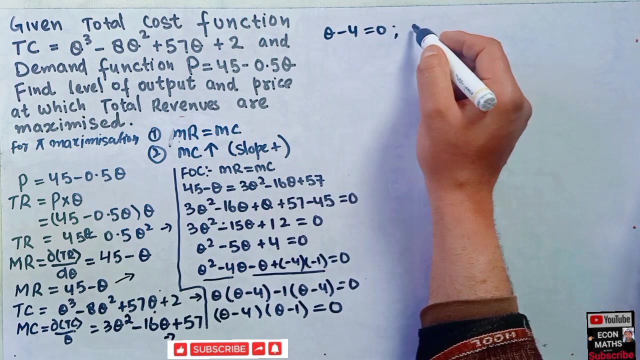 minus 4 and q minus 4. out q minus 4 and q minus 1, this should be equal to 0. I hope I am making myself clear how to solve the quadratic equation. now solving further, that means our q minus 4 should be equal to 0, or our q minus 1 should be equal to 0, or q is. 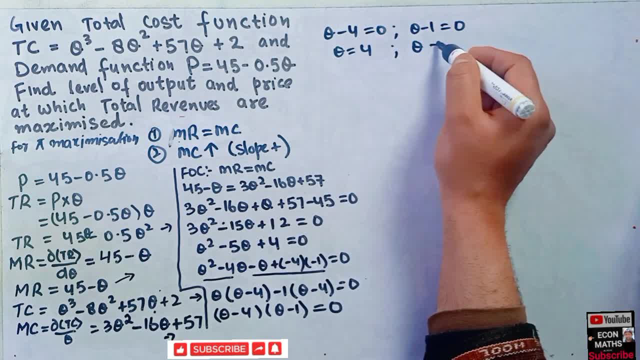 equal to 4 or q is equal to 1. so we get two values of quantity, that is, q is equal to 4 and q is equal to 1. okay, we have to see which of these two levels of output maximizes our total revenue for that. 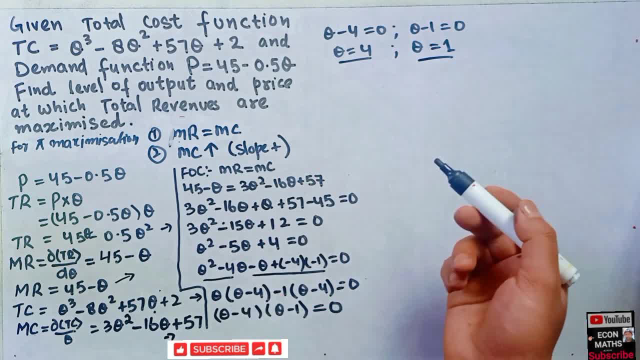 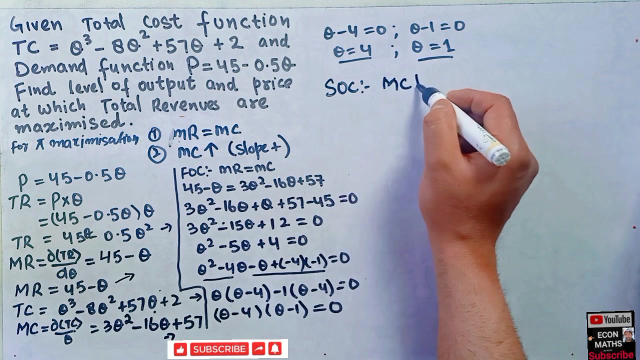 we use the second order condition now. second order conditions tells us, so I will write. second order condition tells us that at the intersection of marginal revenue and marginal cost, okay, the marginal cost should be rising, that is, our marginal cost should be rising, or the slope of the marginal cost should be positive. so I will. 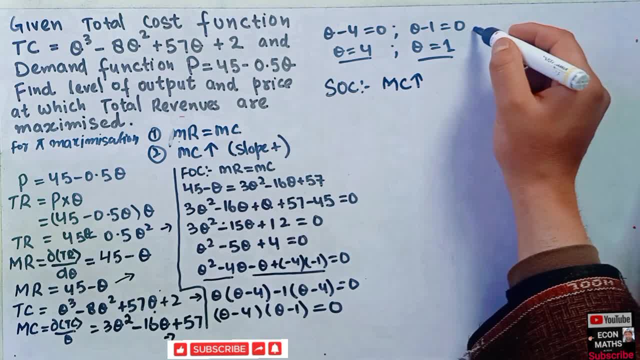 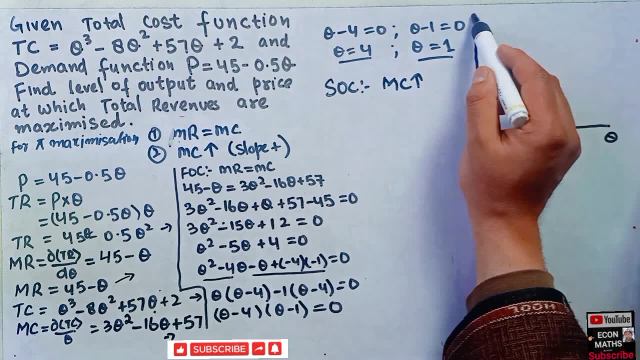 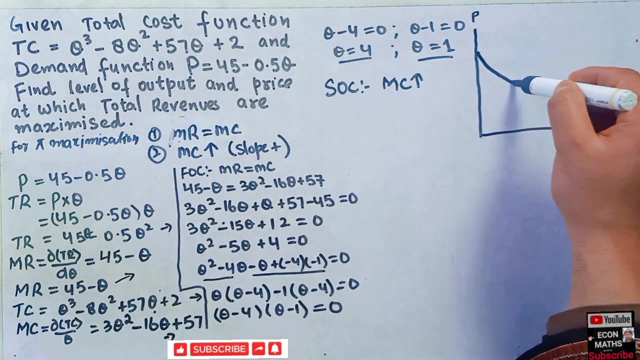 make you it clear by making a diagram. so let us say we have quantity on this axis, price, marginal revenue, marginal cost on this axis. so let us say this is our marginal cost curve. okay, which we got. let us say: this is our marginal revenue curve, this is our marginal revenue curve. so 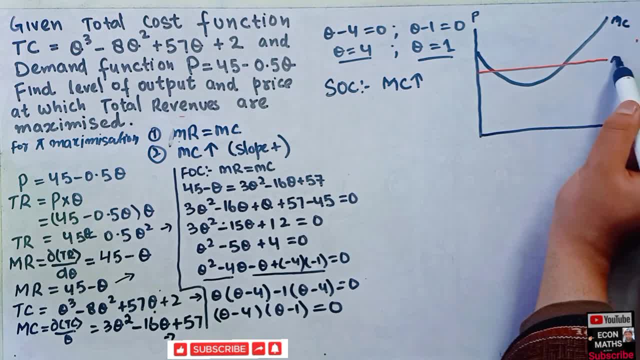 this is like right here. this is marginal revenue. now, first order condition requires that you should think of that as here料. marginal revenue should be equal to marginal cost. so at this point we have: marginal revenue is equal to marginal cost. at this point also, we have the 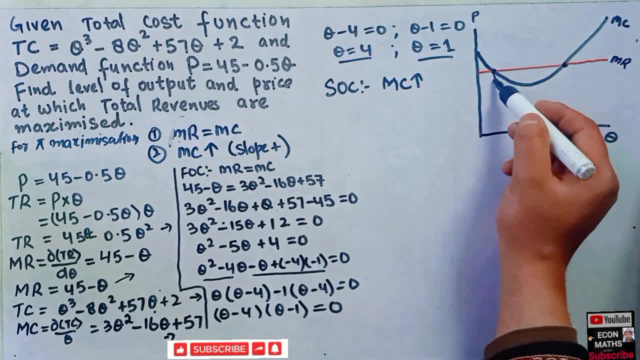 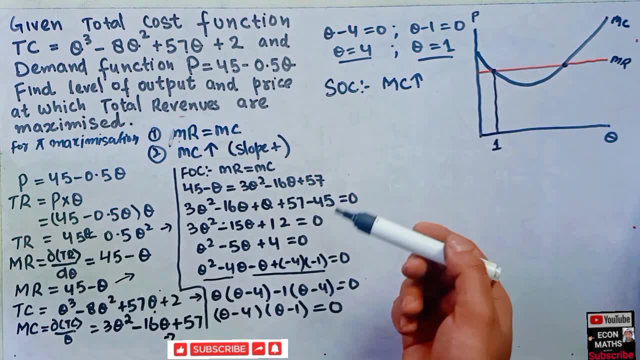 marginal revenue is equal to marginal cost. okay, at this level, that is, at q is equal to one, marginal revenue is equal to marginal cost. so first first condition is satisfied here. also at this point, first condition is satisfied when q is equal to four. okay, so we have to say which of these two level of outputs maximizes the total revenue. for that we use the. 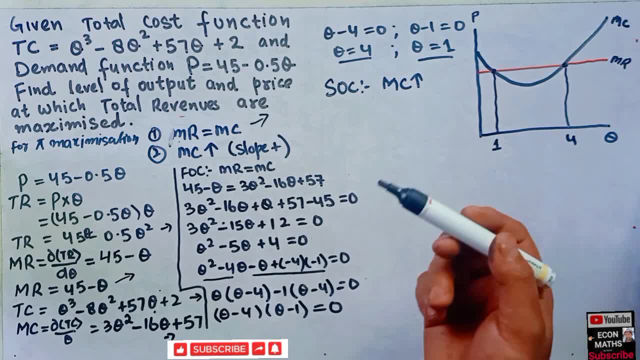 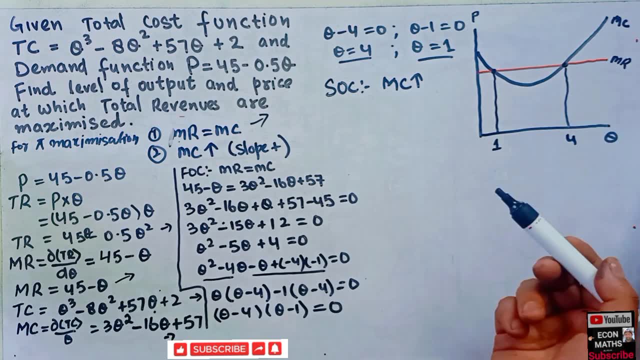 second order condition. second order condition tells us that the slope of the marginal cost should be positive at the intersection of modern revenue and modern cost. okay, so here we can see: the slope is negative at this point. the slope is positive. okay, so this is demographic explanation of um how, how to find the profit, or rather the revenue maximization, output level and price. okay, 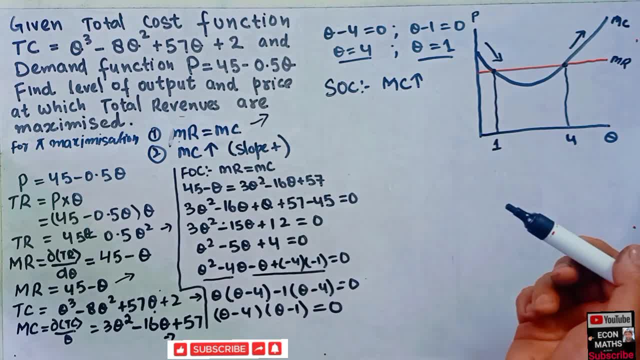 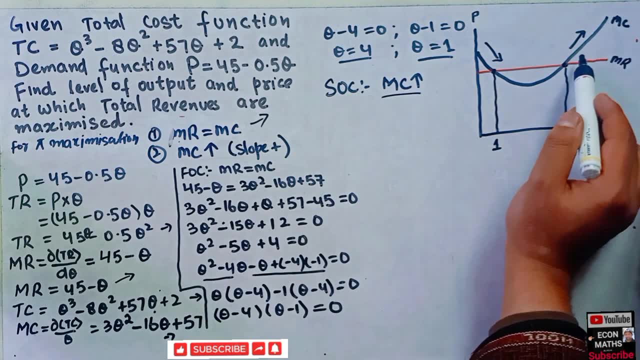 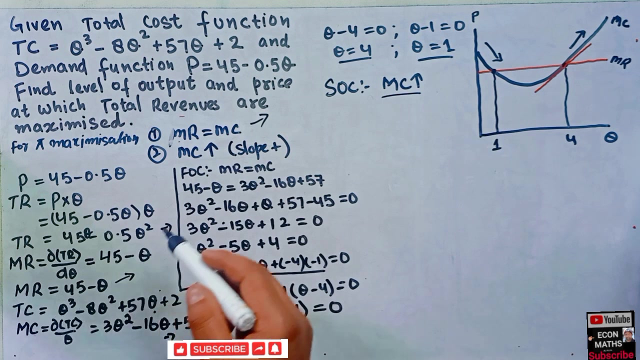 so after that, why? what will we do? we will see what is the slope of the marginal cost. this is our marginal cost. now, to find the slope of the marginal cost, we have to differentiate a marginal cost function. uh, with respect to, with respect to quantity, our marginal cost was somewhere. this is our marginal cost function. 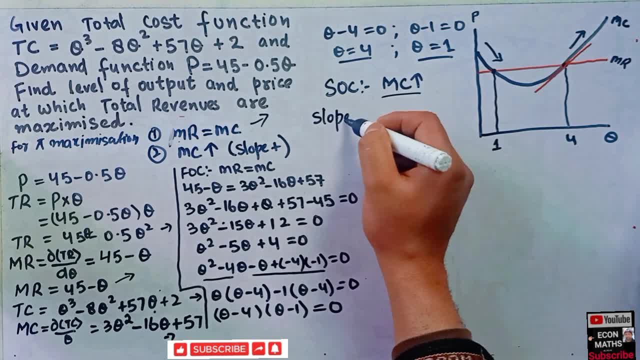 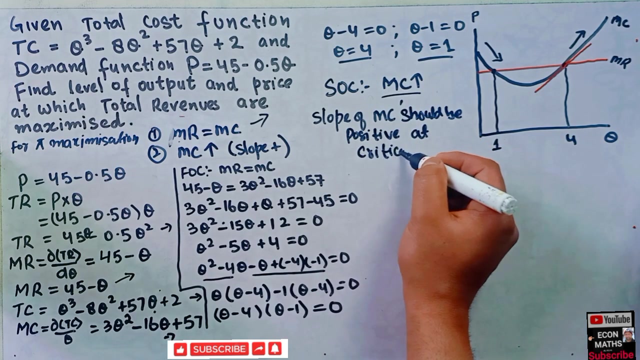 now slope of uh, slope of marginal cost should be, uh, should be positive, so i will write it here: should be positive at critical pointers. by critical pointers we mean the point. we mean the point is of q is equal to 1 and q is equal to 4.. 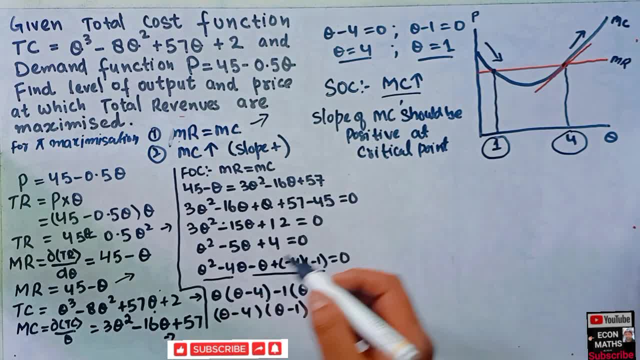 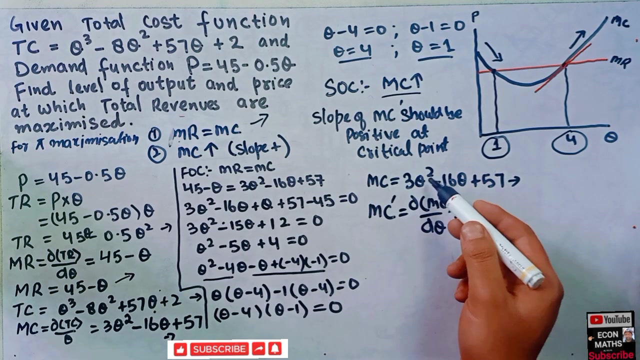 now this is our marginal cost function. so i will write: marginal cost function is 3 q square minus 16, q plus 57, now differentiating this marginal cost function. so i will write here: marginal cost, that is mc prime is equal to d m c divided by dq, which is equal to now three twos are six q. 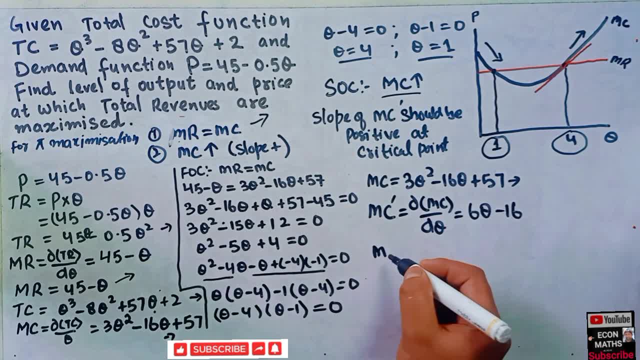 minus 16.. so the slope of marginal cost- i have denoted this by this mc prime- is equal to six six q minus 16.. now we have to insert the value of the critical points and and see whether we get the positive number or negative. if we get the positive number, 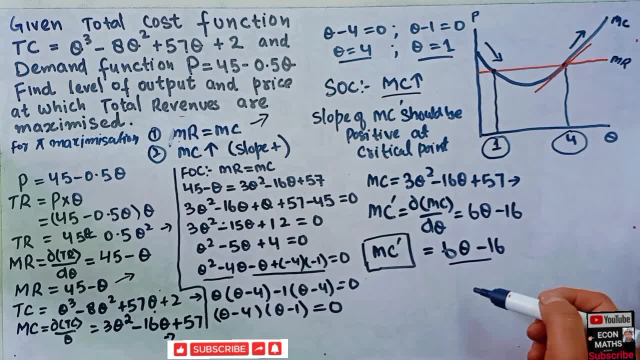 here, then the output is maximized at that, at that critical point. now, when mc prime, when q is equal to 1, now inserting the value q is equal to 1, this is 6 into 1, is 6 minus 16. here we can see: 6 minus 16 is 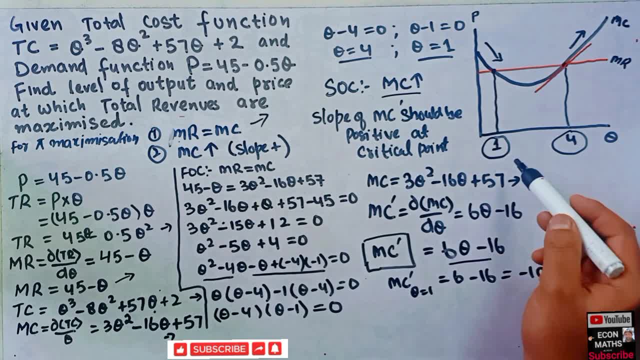 minus 10, which is less than 0. so when q is equal to 1, our revenue will not be maximized. now, giving minus 13 plus 1, this is one zero. so this means j and omega is going to go five to one, so 0 minus. 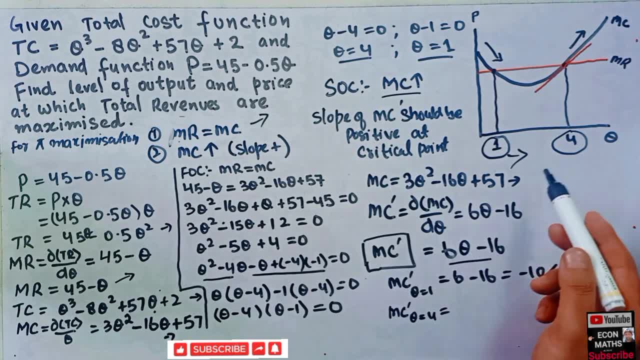 10 plus one is um 0, which is greater than zero. so from this i will write here: uh, 4. now let us. this is equal to 0 and this is 0 and same. here, and um is equal to thing. this is equal to that zero. here we are indicating that j is equal to 5, 2 j and omega are equal to. 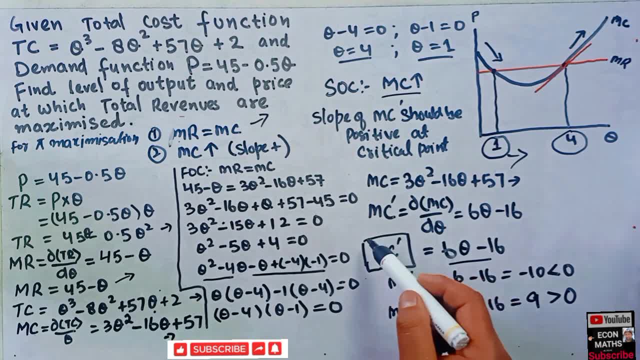 0 plus 5. so now, filling this up, we can see the following: that this value, q, is equal to, q, is equal to 3, d, and when q is here, this is also a peak and, as you can see, q is a mentor of a sum. we can see that consists of mc. when we have this such 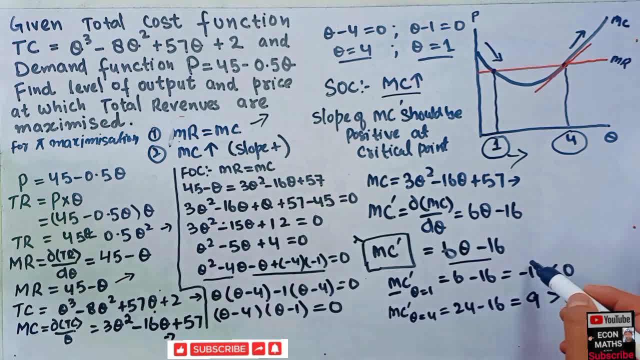 is the value q is equal to 1, q is equal to Comme from here, which is greater than 0, so this i have to 1. our slope is minus 10, which is negative. so this q is equal to 1 will not maximize the total revenue. when q is equal to 4, the slope of this marginal cost curve. 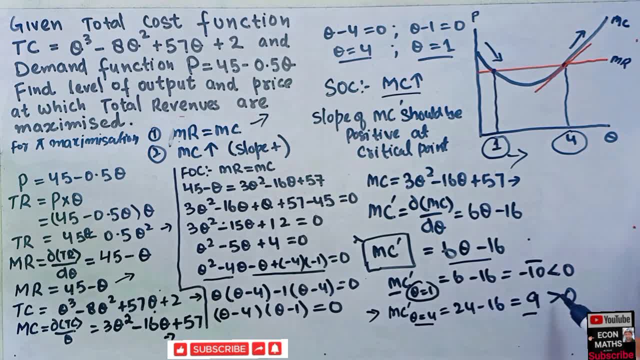 is 9, let us say it's 9, so we see here the, we get here the positive number, so we can say that this q q is equal to 4. this output level will maximize the total revenue. okay, uh, i just want to repeat here. there are two conditions for.